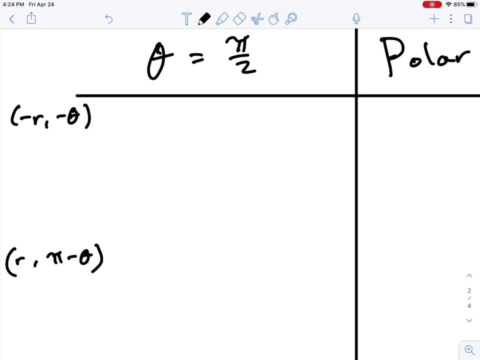 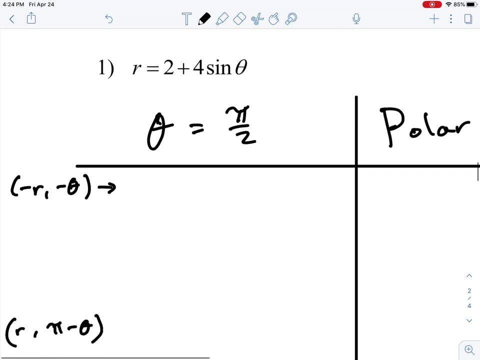 other words the supplement. If, by replacing r and theta with either one of these, we should end up with what's called an equivalent equation. And let me be really clear about the equivalent equation. Ideally, our equivalent equation will be exactly the same as our original equation: r is equal. 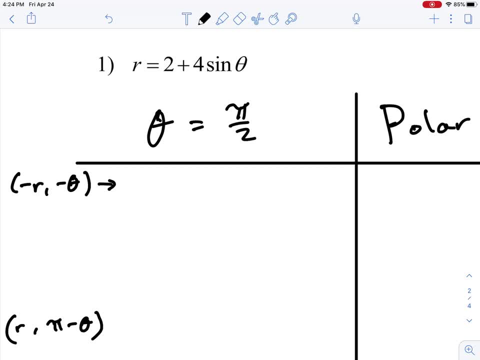 to 2 plus 4, sine theta. So if we end up with that, then we're golden. We know that they're equivalent equations. There are going to be times, however, where we don't get that, And if that is the case, we're likely going to have to just use the other two equations. 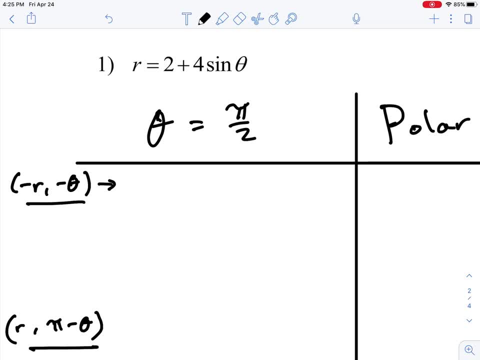 So if it's not this one, it means it's this one. Hopefully it's both, But if it's not one, it's the other. And what this is really saying is there are polar equations that are not the same, meaning they don't look the same, but they actually produce the same polar. 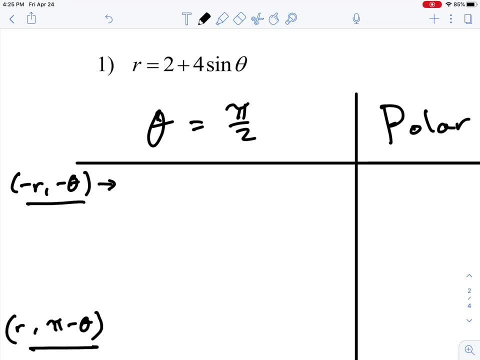 graphs And we would still consider those equivalent equations. So what we're looking to find are equivalent equations, And it's hard to tell just by looking at these, because we're not really experts on polar graphs yet. So that's something to consider when looking at these equations. And then it's also really going to be about 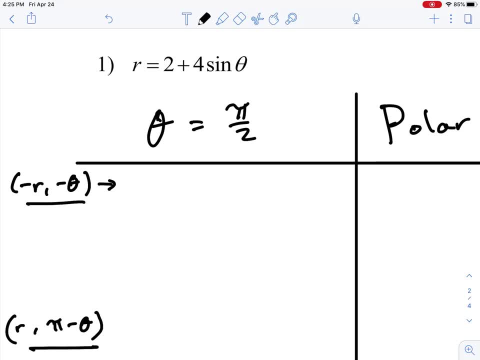 measuring the reason for these and also looking at some of the other equations, And so that's really important. so that's one way to see these coming together, But also we're looking to why we're going to take a little bit more work to check them algebraically. So let's start with this. 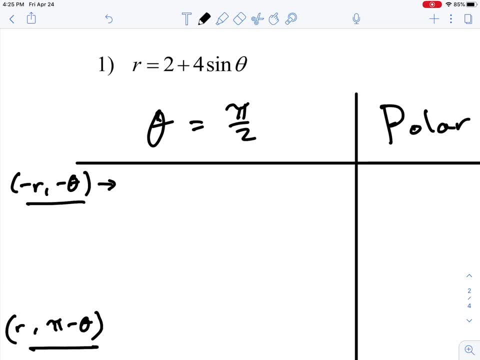 first one and then hopefully it'll make more sense as I start going through some of these practice problems. So the first equation, r equals 2 plus 4 sine theta. we're going to go ahead and replace the r and that theta with negative r and negative theta, which would give us negative r. 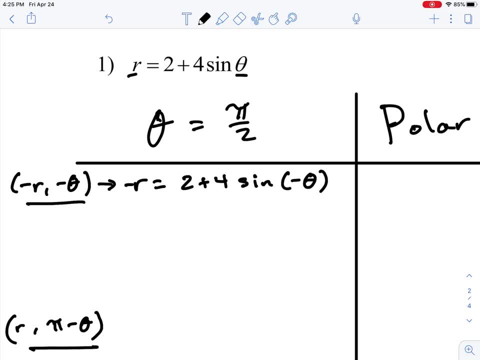 is equal to 2 plus 4 sine of negative theta. So if I were to just clean this up a little bit here, I'm going to go ahead and divide everything by negative 1.. So r is equal to negative 2 minus 4 sine of negative theta. And at this step here we're going to want to use our 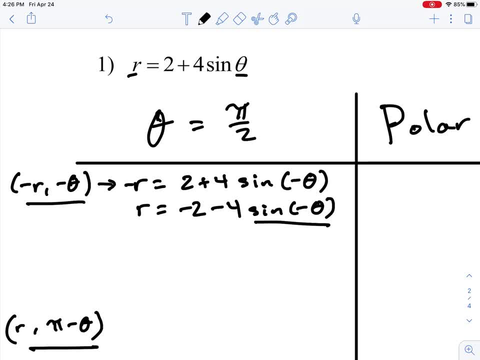 even and odd identities. We know that sine of negative theta is equal to negative sine theta because it's an odd function. So we can rewrite this as: r is equal to negative 2 minus 4 times negative sine theta. And if I clean that up even further, we can say: r is equal to: 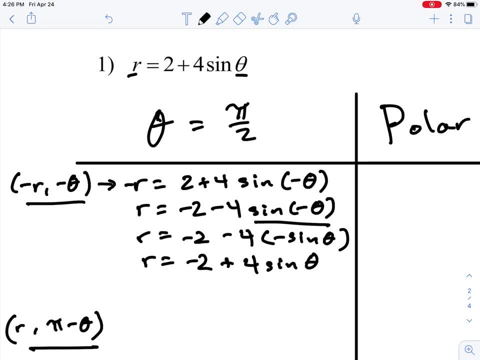 negative 2 plus 4 sine theta. So I'm going to pause here for a second. compare this to our original equation: r is equal to 2 plus 4 sine theta. we can see here that they're clearly not the same. Well, we don't know just yet again because we haven't worked too much with polar. 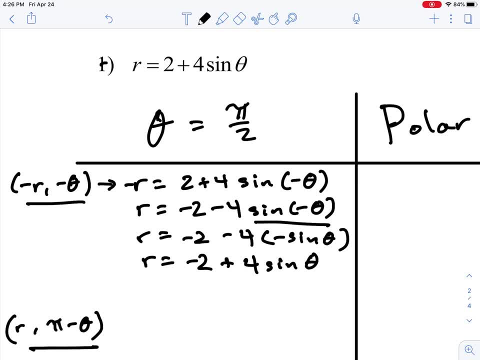 graphs is whether or not these are equivalent equations. Meaning, do these two equations that we have here do they produce the same polar graph? and it turns out they actually do. but we wouldn't know, know that and we're gonna that, we don't know that, and so right now we're going to say: so far, it looks like it doesn't work. 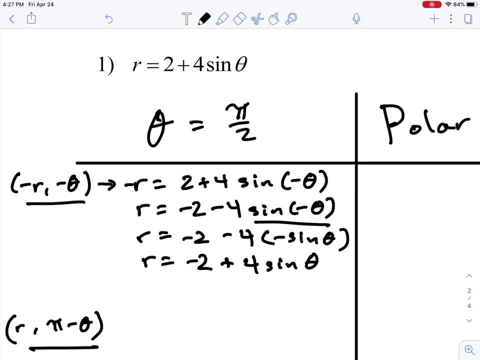 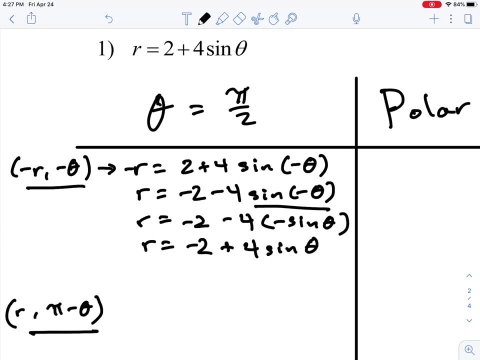 that these are. these don't appear to be equivalent equations. even though they are, they don't appear to be equivalent equations because they're not the same. so that leaves us really with no other choice but to check our second option, or second waves, seeing whether or not it is symmetric with 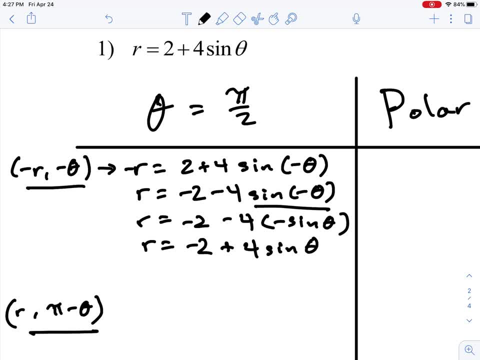 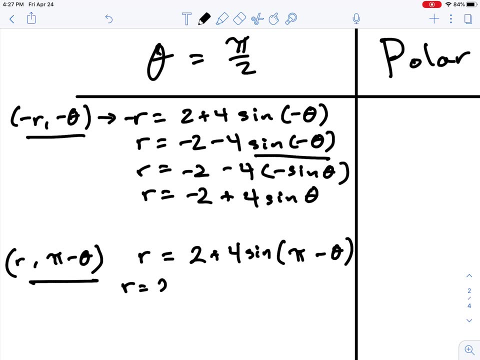 respect to pi over 2, and that's to replace our angle theta with pi minus theta. so we're going to go ahead and write: r is equal to 2 plus 4, sine and again replace theta, this time with pi minus theta, and what we're left with here is the following: r is equal to 2 plus 4, and you might be. 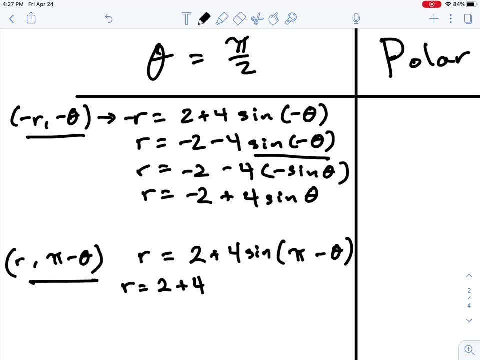 wondering how to evaluate that and i'm going to ask you to kind of think back, think back, think all the way back to. you guessed it- sum and difference formulas. so we're going to write this now as the sine of theta cosine of- excuse me- sine of pi- cosine of theta, minus the sine of theta cosine of pi. 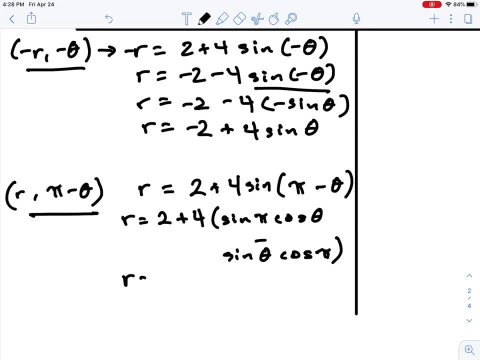 you remember that? i'm sure you all do so. r is equal to 2 plus 4, and let's go quickly evaluate this. sine of pi would just be equal to 0, so that first term completely becomes 0. cosine of pi becomes negative 1, so negative 1 times sine of theta. 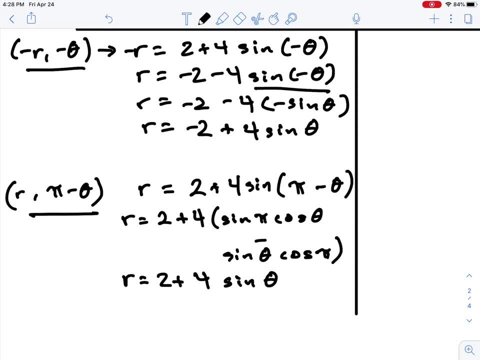 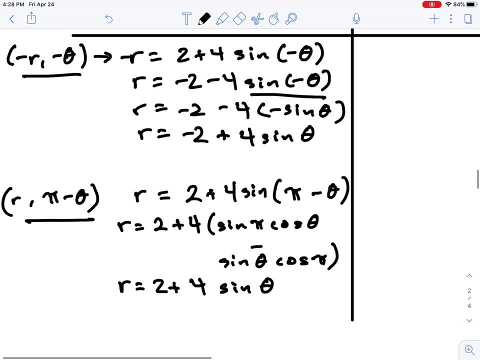 we can just write this as sine theta. and what do you know? we notice here that we do get the same exact equation as what we had originally. so this verifies that we do have an equivalent equation. so we can go ahead and write this: it works there. it doesn't seem like it works there. 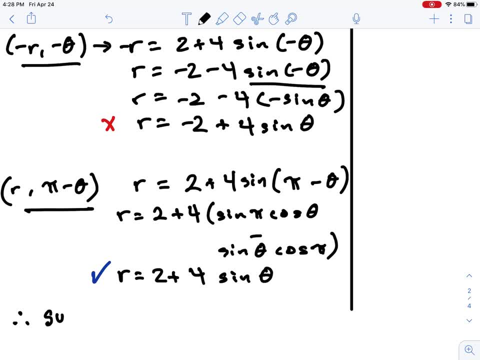 but it doesn't matter. if one of the two checks work, then we know, we can say: therefore it's symmetric with respect to theta is equal to pi over 2. okay, and again, if i were to graph both of these two equations, i would see that they produce the same polar graph, so technically they have equivalent equations. 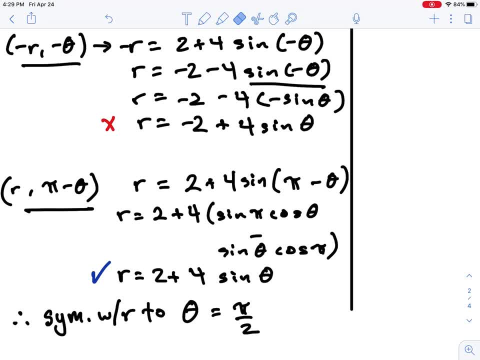 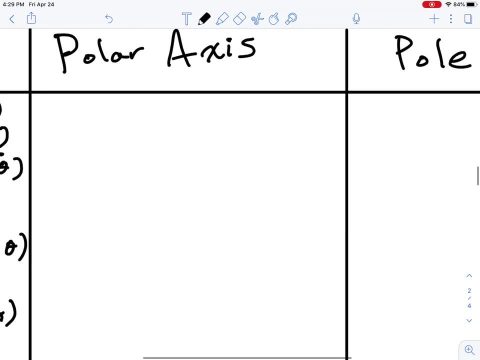 but for now let's go by checking algebraically and saying: hey, i know that the first check didn't work, but the second test did. therefore it's symmetric with respect to pi over 2. okay, all right, now let's try the next act. uh, the next one, the polar axis. so for the polar axis, remember the. 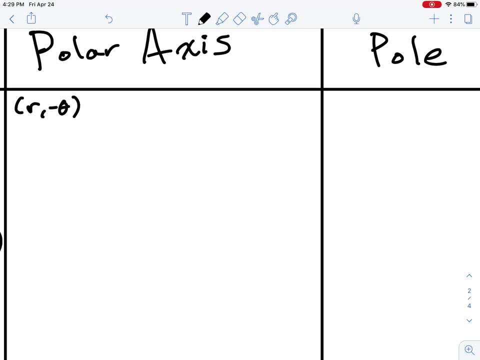 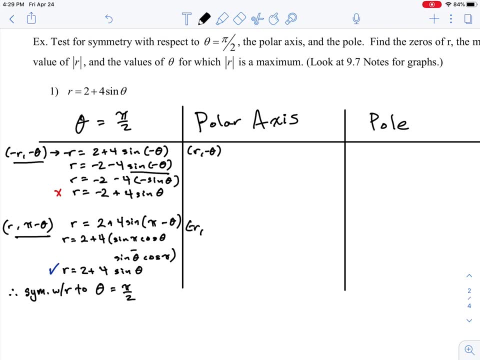 two checks here are the same, so we're going to write this as sine of theta and let's go ahead and check here. we can replace r and theta with r and negative theta, or we can also check by writing r- excuse me- negative r, pi minus theta. so let's check to see if either one of these 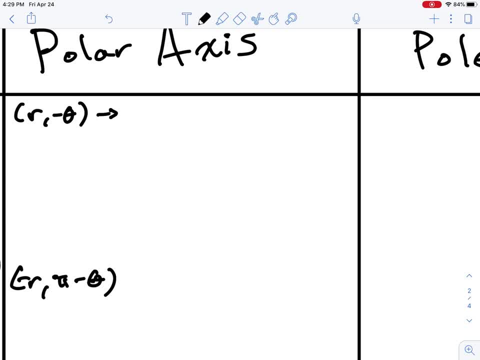 two work, so let's go back. so for the polar axis, we're going to say, replacing theta with negative theta gives us 2 plus 4 sine of negative theta, and this is a quicker check: 2 minus 4 sine theta. and this one clearly does not seem to work. okay, so let's try the other. 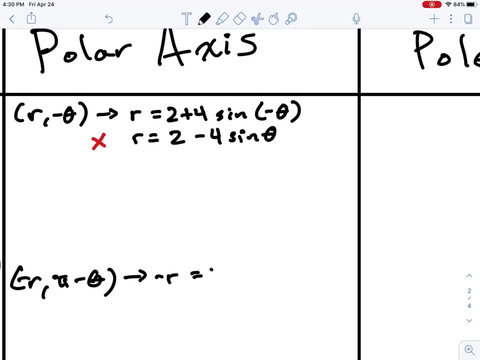 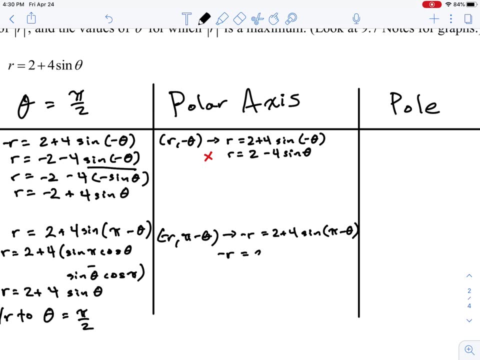 one. so now for the other one. here we're going to say: all right, let's replace r with negative r, 2 plus 4 sine pi minus theta. and we already did the heavy lifting for 4 sine pi minus negative theta. so we can just write this: as negative r is equal to 2. 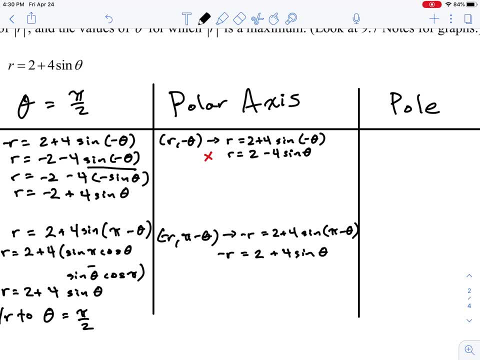 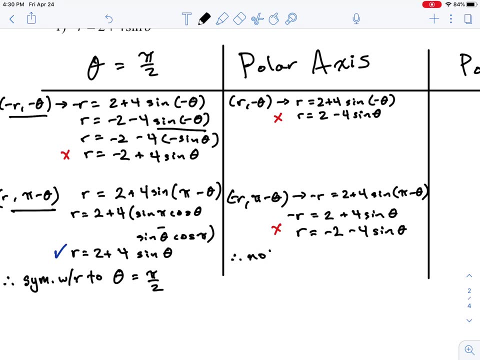 again. this would just all of this would just come out to plus 4 sine theta, and divide everything by negative r. now r is equal to negative 2 minus 4 sine theta. in any sense we see that these are not the same equations, so we can go ahead and just say: therefore not symmetric. 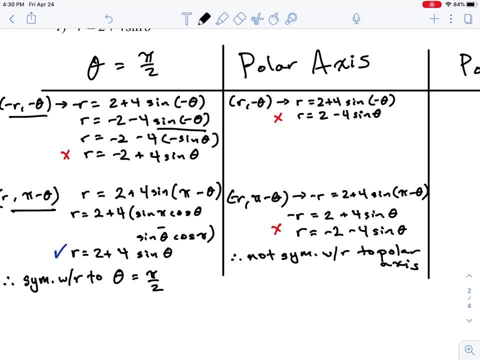 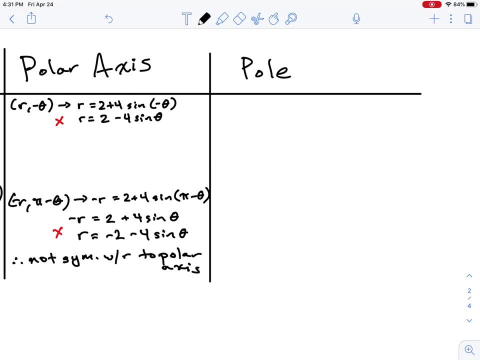 with respect to the polar axis. okay, all right. now the last check is to go ahead and see if it's symmetric with respect to the pole. so there are two ways for that. we can either replace r theta with negative r positive theta, or we can go ahead and check to see. 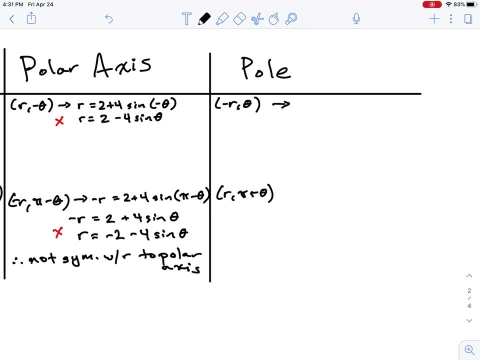 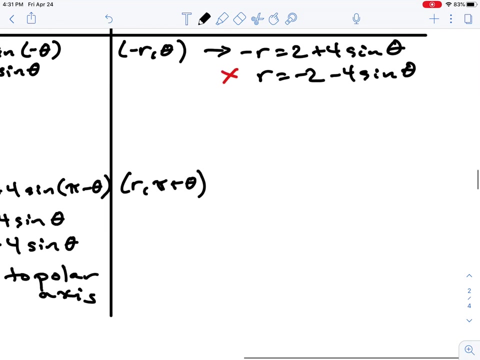 if this works. so by replacing r with negative r, we would get negative. r is equal to two plus four sine theta, which is, which is just, r is equal to negative two minus four sine theta, not the same. so this one does not work. Now, replacing r or, excuse me, theta with pi plus theta, let's check in on this one. 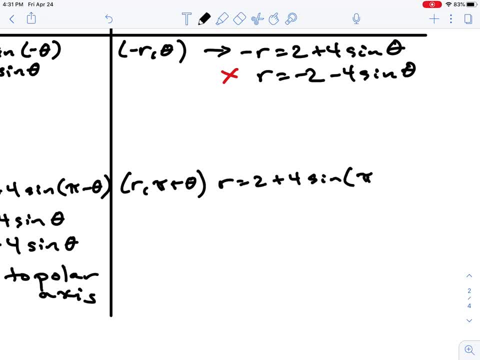 So we would say r is equal to two plus four, sine pi plus theta, so r is equal to two plus four, and then again we're gonna have to use the sum formula for sine, which is just sine theta, cosine, excuse me, sine pi, cosine, theta plus sine theta, cosine pi. and a quick evaluation of this. 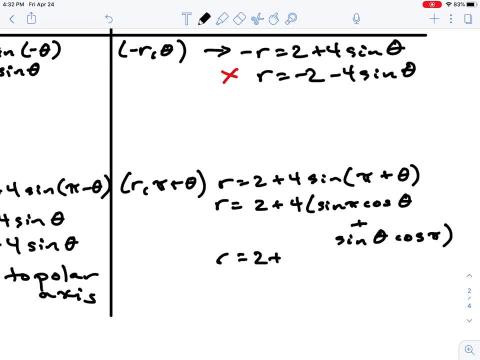 we see r is equal to two plus sine of pi is equal to zero. so again all of this becomes zero. Cosine of pi is equal to negative one. so we would actually have negative four sine theta as our result, and this also is not the same. so we can say therefore: 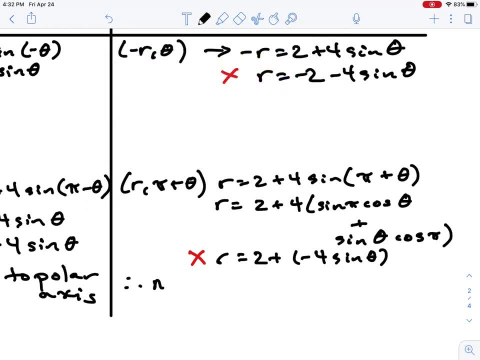 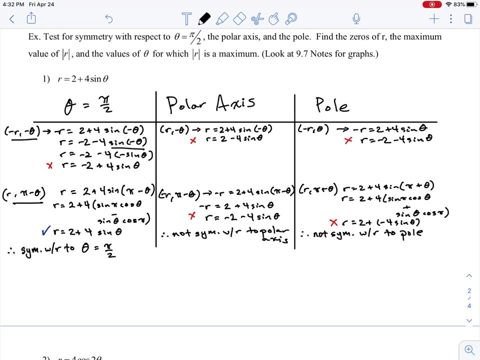 this is also not symmetric with respect to the pole, and let's write that Therefore not symmetric with respect to the pole. So the only symmetry that we were able to verify algebraically was that this polar graph is symmetric with respect to the angle. theta is equal to pi over two. 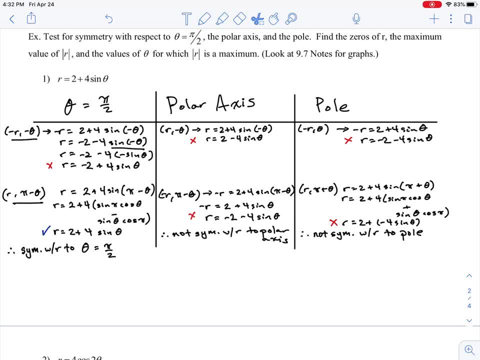 and if I were to go ahead and let's see if I can just go back to that original graph, and it looks like it's not symmetric with respect to the angle, theta is equal to pi over two and it looks like I don't have it anymore. but if you recall that graph, it was a Limasson. 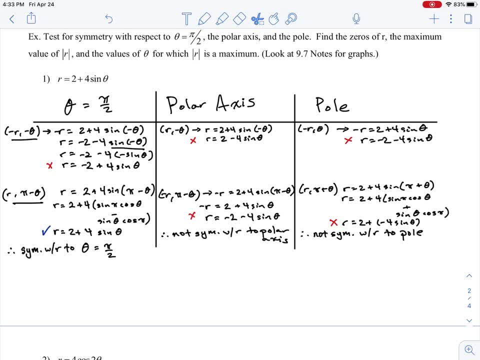 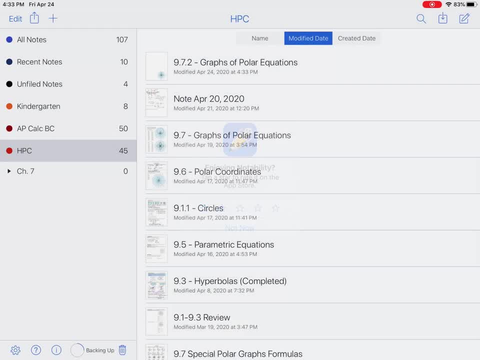 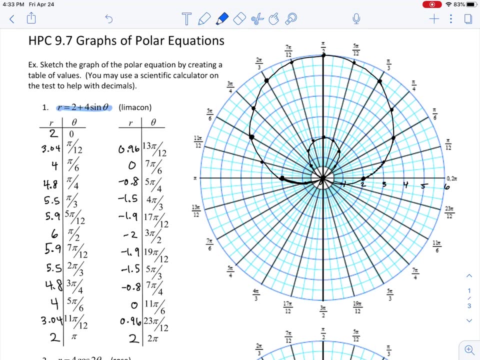 Just look back to your notes from part one, or just what we did early on in 9.7.. It's the very first graph We see that it is actually. I can just reference it here real quick, Not that I don't care about reading you right now. There's our Limasson, There's our graph. 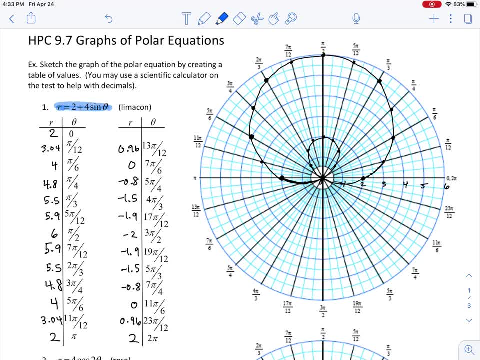 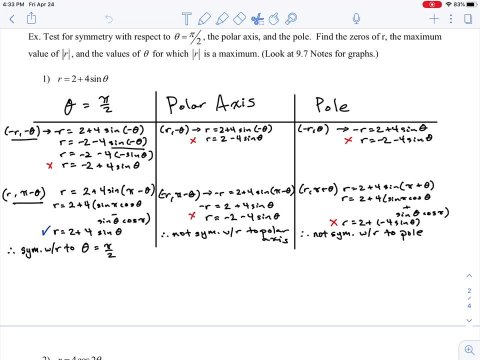 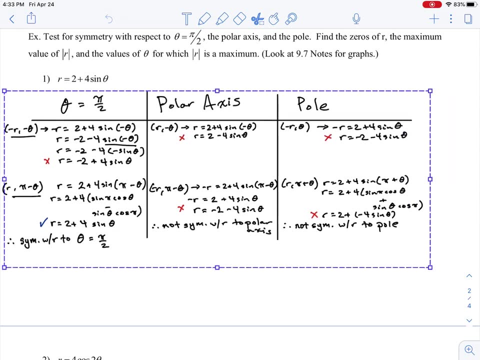 two plus four, sine theta, We see that it is indeed symmetric over pi, over two, and not anything else. So let's finish up that problem now by actually going ahead and talking about finding the zeros and the maximum values. So let me go ahead and make this a little bit smaller, so we have a little bit. 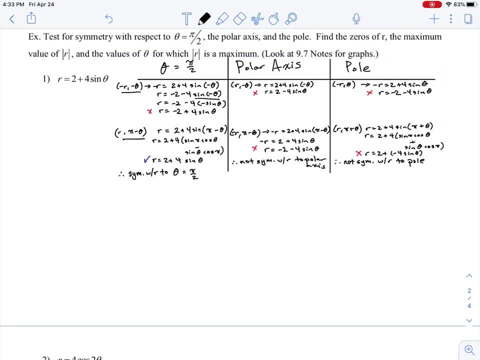 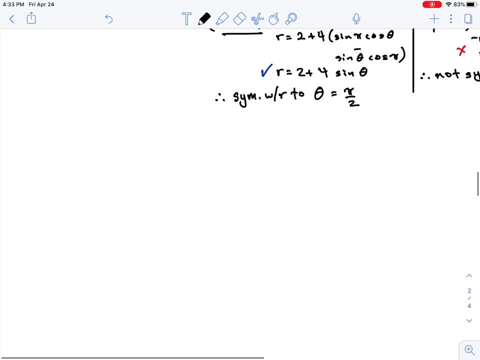 of space to work with. I can make this a little bit bigger later, but I'll just move this off to the side for now. Okay, so let's go ahead. and now let's check for our zeros. So, to find the zeros. 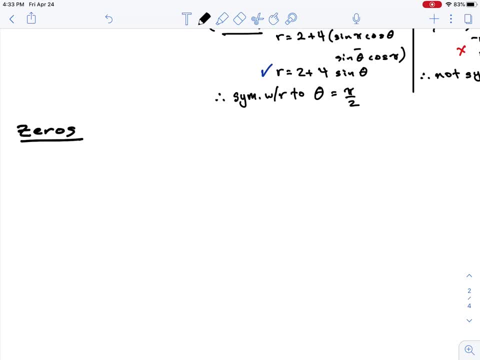 and again make sure we're clear about what we're talking about when we're finding the zeros. The zeros of a polar equation are the values of theta where r is equal to zero. Again, the values of theta where r is equal. 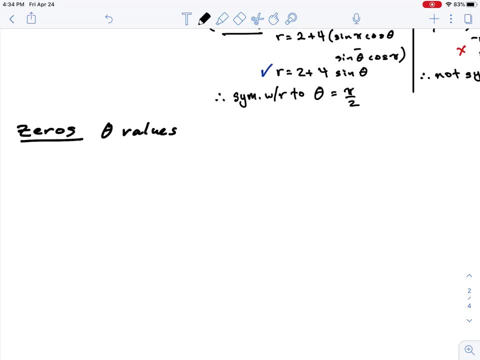 to zero. So it's the theta values where r is equal to zero. So all that means is, just like when we found zeros of regular rectangular equations, we're going to set our polar equation equal to zero. So zero is equal to two plus four sine theta. Well, just doing some. 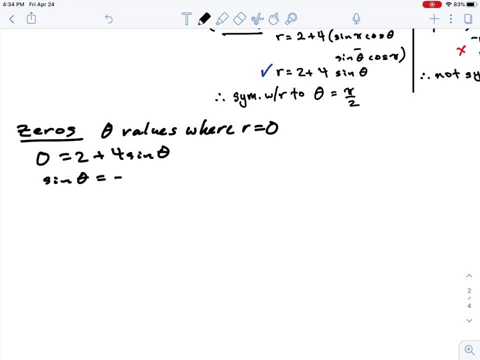 quick solving. here we're going to write this as sine of theta is equal to negative two-fourths or negative one-half, And just like we did when we solved trigonometric equations, you're asking yourself: okay, what are the angles of theta that give us negative one-half here? that give us 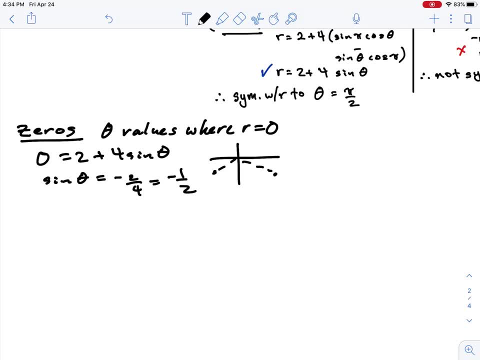 negative one-half. So what values of theta give us negative one-half? Well, theta would have to be equal to seven pi over six and eleven pi over six, Because we all remember our unit circle right. All right, So those are our zeros. Those are the values for theta, so that r is equal to zero. 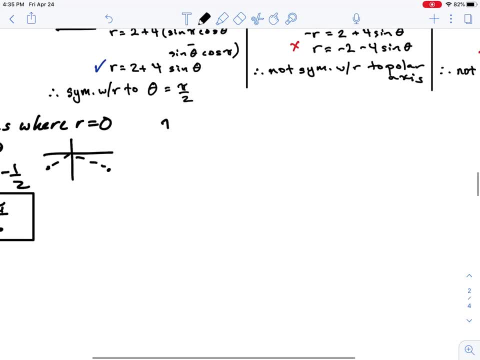 Now let's go ahead and find our maximum values for r. So the maximum r values here? okay, Maximum absolute r values. So again we're going to write this as sine of theta, where r is equal to zero. Again, for our polar equation, r is equal to two plus four sine theta. ask yourself: 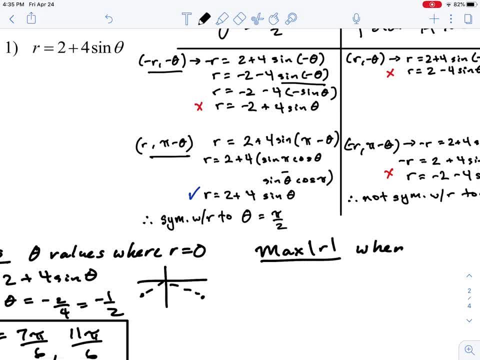 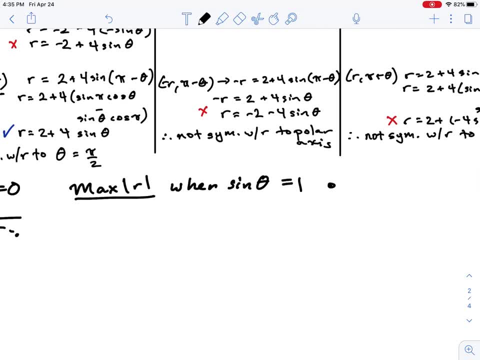 the maximum value is going to occur when sine of theta is either equal to positive one or sine of theta is equal to negative one. So let's consider both scenarios here. So what would happen when sine of theta is equal to one? Well, when sine of theta is equal to one, so r is equal to two plus four sine theta. If all of 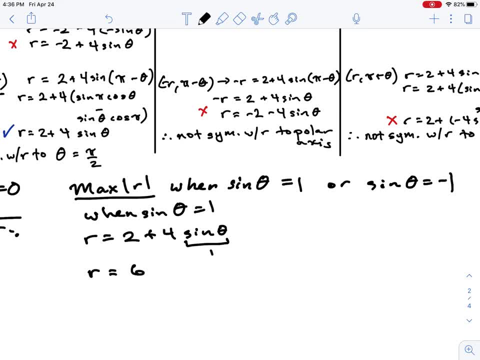 this were equal to one, then r would just simply be equal to six. When sine of theta is equal to negative one, r is equal to two plus four sine theta. If all of this is equal to negative one, then r is equal to negative two. 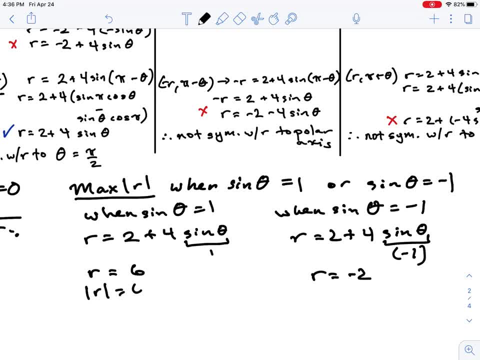 But we're looking at the absolute value of r here. So the absolute value of r is equal to six. The absolute value of r here is equal to positive two. So which one is the larger value? Well, clearly, six is greater than two. So we say that the maximum value of r here is six. So now we can. 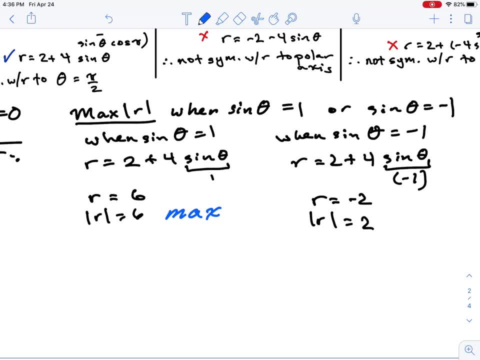 finish this off by asking ourselves: okay, so, since I know that maximum r value is six, when does that occur? That occurs when the absolute value of r is equal to two. So we say that the maximum value of r occurs in this scenario. here The max occurs when sine of theta is equal to one. Well, to finish, 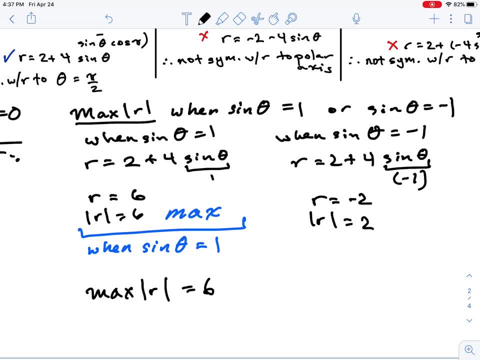 this off. we can say: our max value of r is equal to six when sine of theta was equal to one or more succinctly, when theta is equal to pi over two. And you might be asking yourself: well, couldn't I have just said I know the maximum occurs when theta is equal to pi over two because 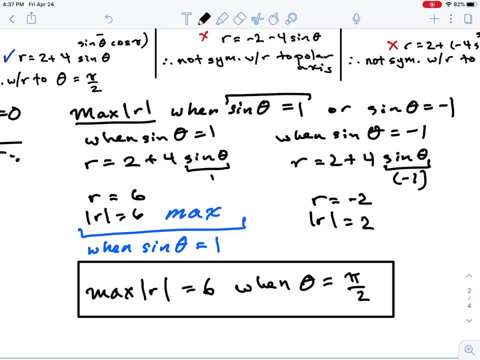 that's when I know sine of theta is equal to one. Well, no, not really, because sine of theta could have been equal to negative one and we wouldn't have known unless we checked. And sine of theta is equal to negative one when theta is equal to three pi over two. So we have to be very clear. 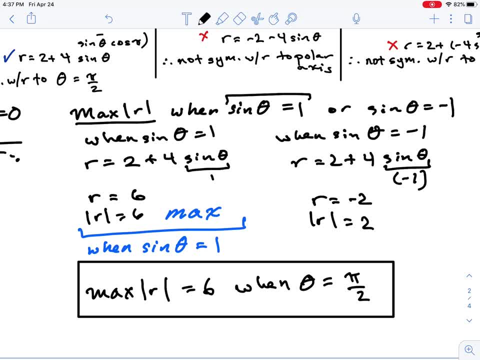 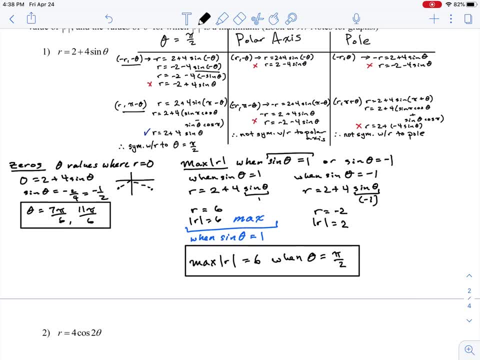 about only selecting pi over two as the angle that produces the maximum, because we know that if we were to try, theta is equal to three pi over two, the absolute value of r. there would only be two, so it wouldn't be the maximum. 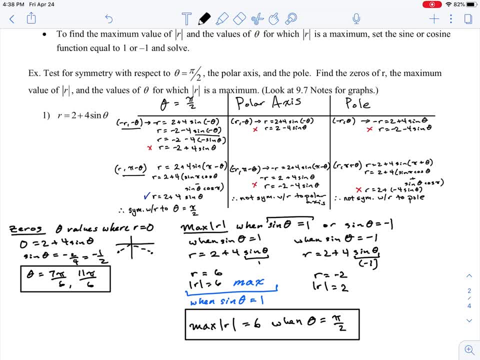 So, just to recap, we went ahead and we tested for the symmetry by looking at its symmetry over pi, over two, the polar axis and the pole- and we were able to find the zeros and the maximum r values. And in the next video I'll just do one more problem, just to make sure that we